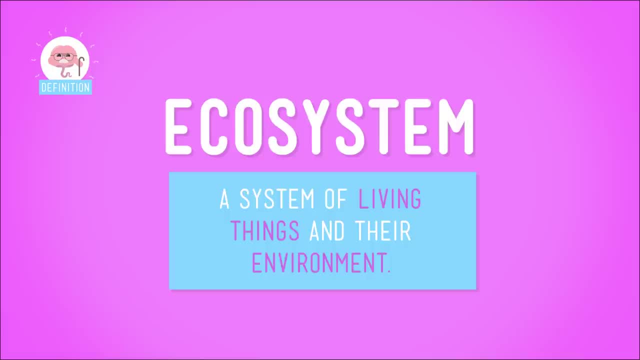 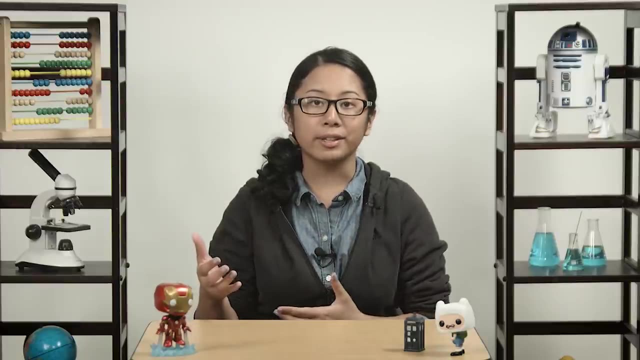 of living and non-living things in a habitat is called an ecosystem. The things in an ecosystem are all connected, Just like when you touch one part of a spider web and the whole thing vibrates. when one link in the food web is threatened, it can. 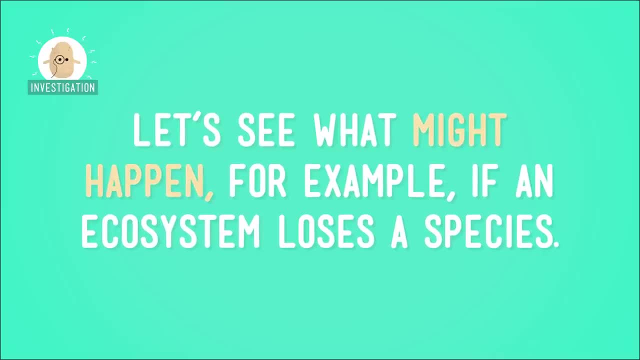 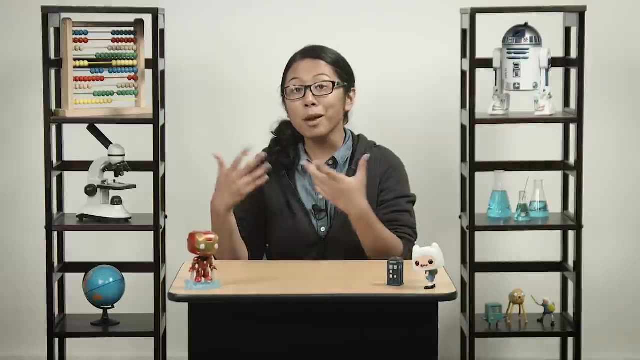 shake up the whole ecosystem. Let's see what might happen, for example, if an ecosystem loses a species. Since we're talking about food webs, I think we should look at spider monkeys. They're called spider monkeys because they hang upside down from their tails with their arms and 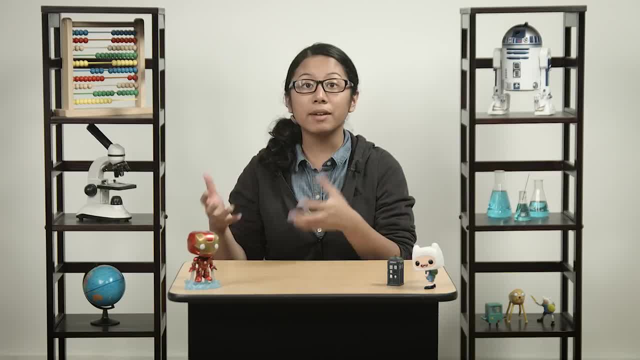 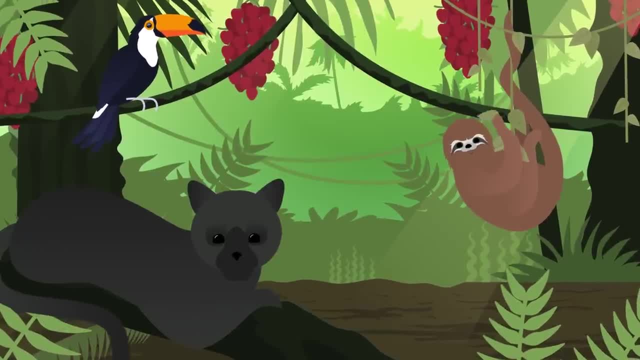 legs dangling. This is somehow completely adorable. These primates live in a tropical rainforest habitat which is just bursting with food. But what about some of the coolest creatures out there: Toucans, Jaguars, Sloths- As we learned last time, these animals need each other to survive- And spider monkeys? 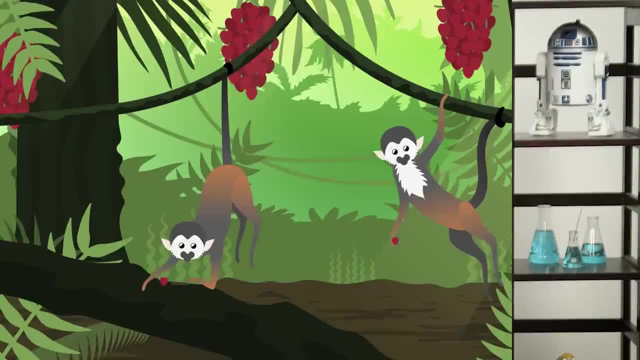 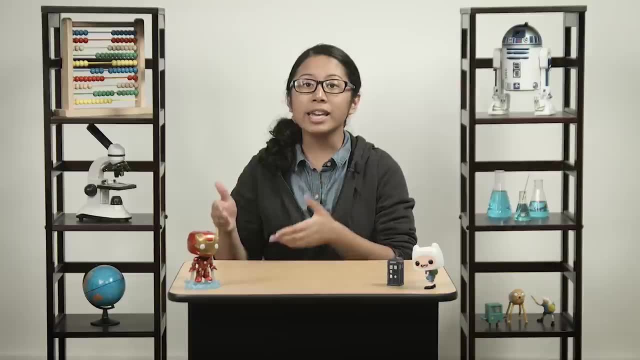 happen to play a particularly important role in the rainforest food web. They eat mostly fruit which contains seeds, and we know that seeds are how plants make more plants. When a spider monkey snacks on a berry, he gets to enjoy the tasty fruit while also doing the plant a solid favor. When the monkey moves on to another part of the forest and um passes the fruit, he leaves the seeds behind. Wait a while, and then what happens? Well voila, You have a new plant. Imagine thousands of monkeys eating thousands of fruits every. 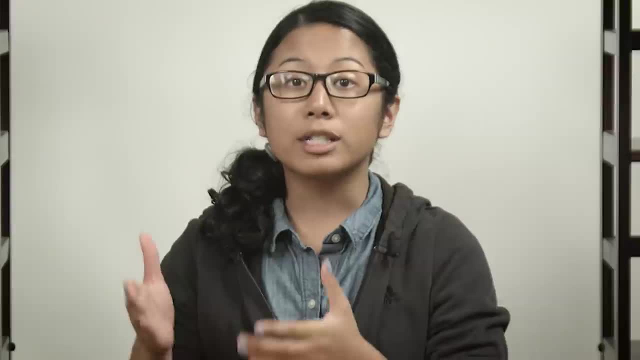 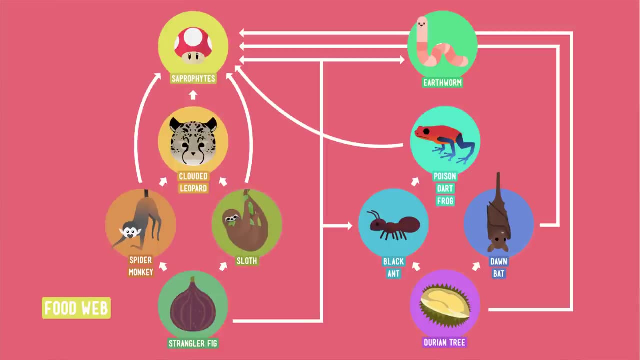 day. More monkeys equals more plants and trees. Those trees support lots of other animals. Insects and sloths eat those plants too, And more spider monkeys, insects and sloths mean more food for carnivores. Leopards dine on the sloths and spider monkeys, while frogs 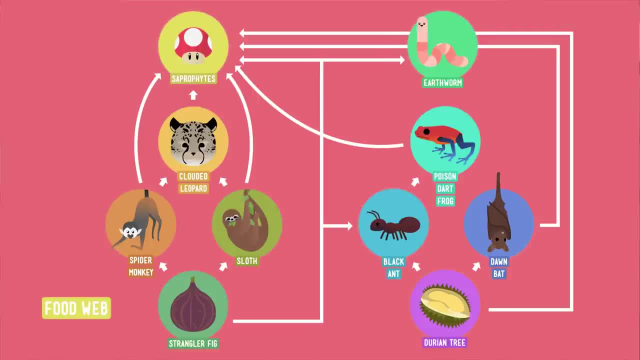 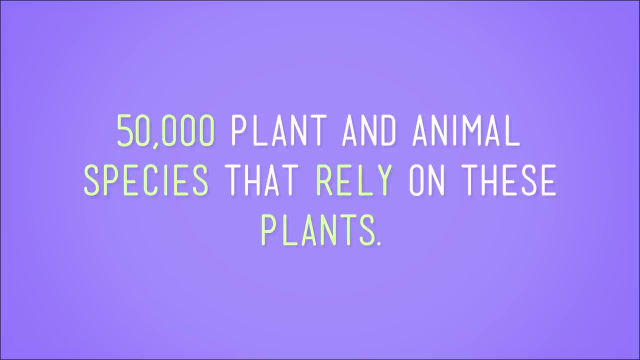 eat the insects And of course, our decomposers, like fungi and bacteria, break down, leftover plant and animal matter. So we're talking around 50,000 plant and animal species that rely on these plants. Now imagine the spider monkey population starts to decline. Maybe they're hit with a strange. 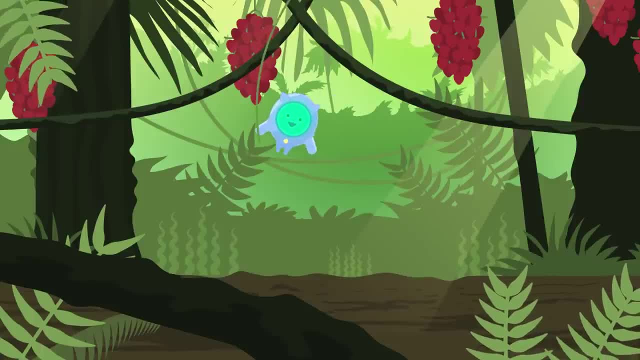 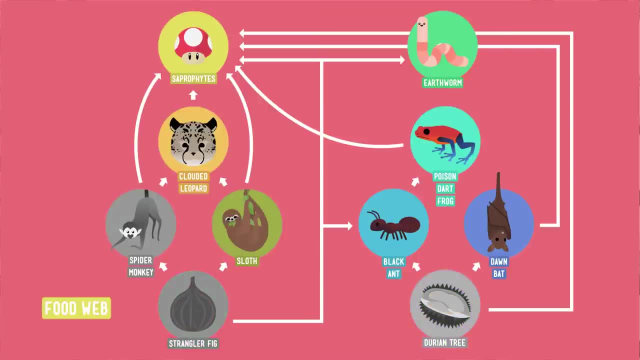 new disease, or maybe humans overhunt them? If the monkeys aren't around to eat the fruit, then the seeds aren't scattered around and the forest stops growing, leaving fewer fruits for fewer monkeys. Not only that, fewer plants means less food for other animals like insects. 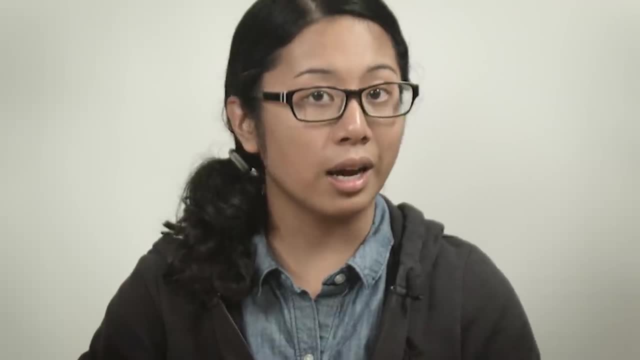 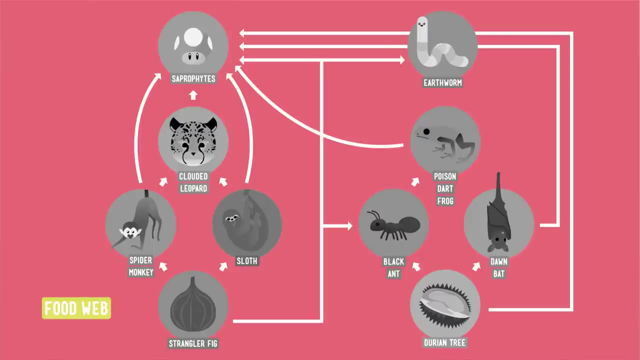 and our sloth friends. That means the insect and sloth numbers start to decline And that means less food for the animals that eat them. All of a sudden, none of the animals in our ecosystem have enough to eat, all because of the loss of one species. 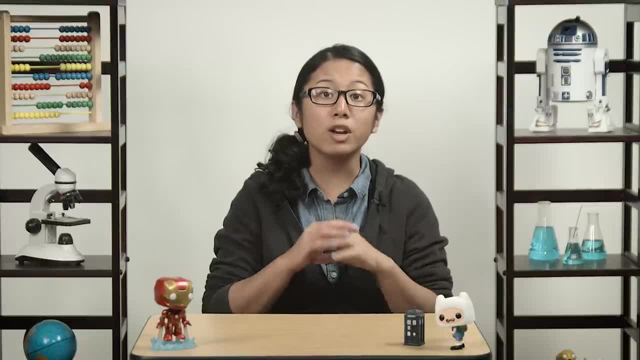 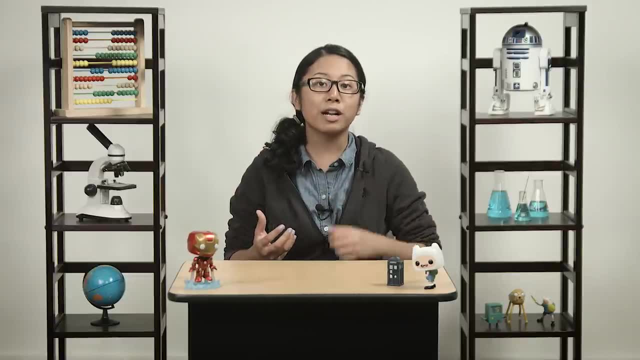 Do you see how this could get really bad? Remove one piece of the food web and you might knock down the whole thing. That's bad news for us too. The good news is that ecosystems want to be in balance After a natural disaster like a forest fire or a flood. things might be wacky for a while, but habitats can usually get back to normal. But if things get really bad, the habitat might change forever. The old species will leave, searching for a better place to live. New species will come in. Life will keep going.